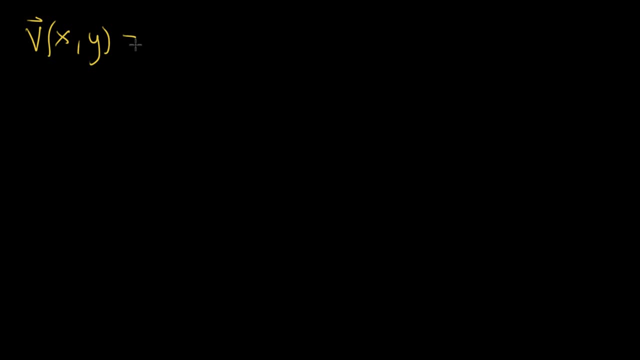 is given by a function that has a two-dimensional input and a two-dimensional output, And it's common to write the components of that output as the functions p and q. So each one of those p and q takes in two different variables as its input: p and q. 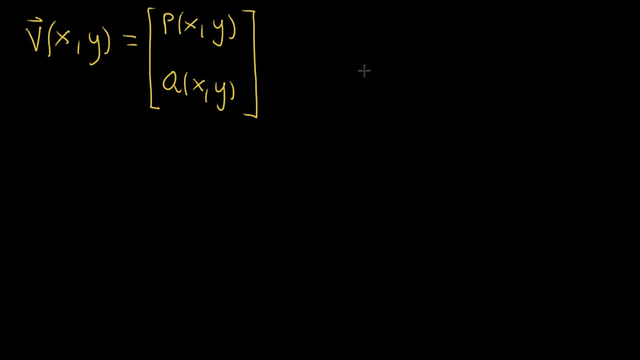 And what I want to do here is talk about this idea of curl- And you might write it down as just curl- curl of v, the vector field, which takes in the same inputs that the vector field does. And because this is the two-dimensional example, 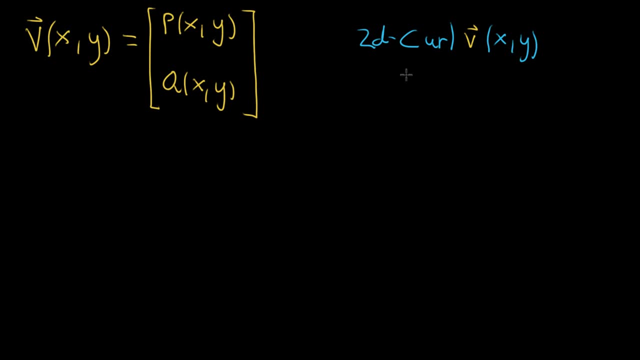 I might write just to distinguish it from three-dimensional curl, which is something we'll get later on, 2d curl of v. So you're kind of thinking of this as a differential thing, in the same way that you have, you know, a derivative e to the x. 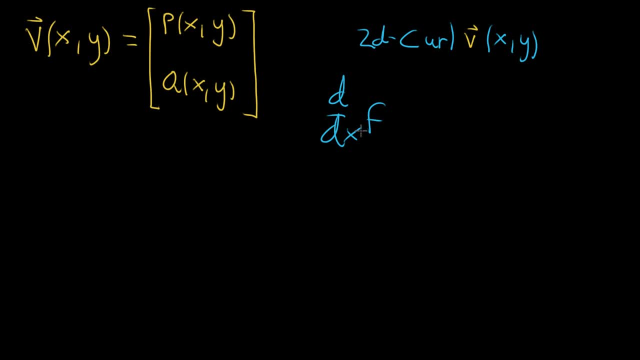 that's going to take in some components. It's going to give you some kind of function And you give it a function and it gives you a new function, the derivative. Here you think of this 2d curl as like an operator. 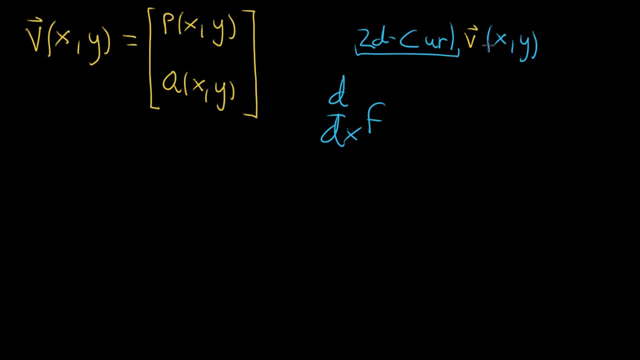 You give it a function, a vector field function, and it gives you another function which, in this case, will be scalar-valued. And the reason it's scalar-valued is because, at every given point, you want it to give you a number. 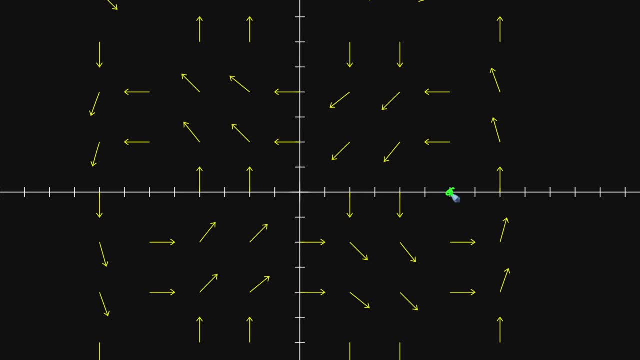 So if I, you know, look back at the vector field that I have here, we want that at a point like this, where there's a lot of counterclockwise rotation happening around it, for the curl function to return a positive number. 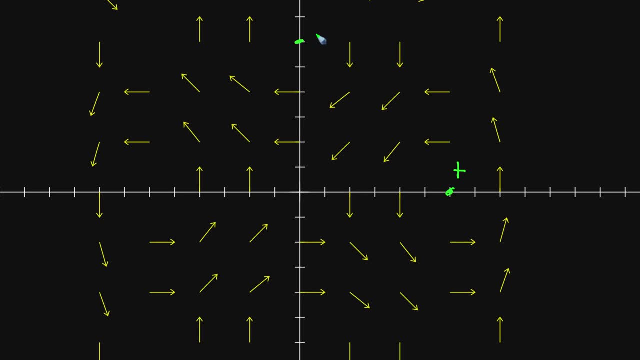 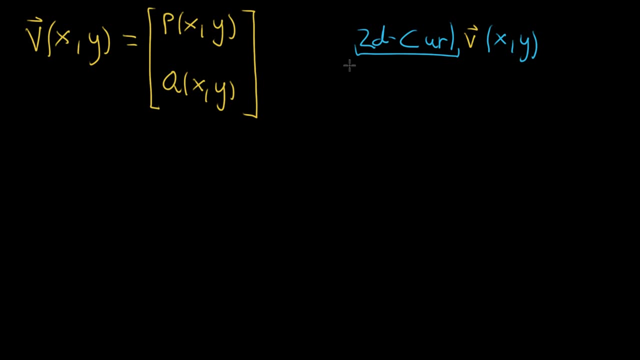 But at a point like this, where there's some counter, where there's clockwise rotation happening around it, we want the curl to return a negative number. So let's start thinking about what that should mean And a good way to understand this two-dimensional curl function. 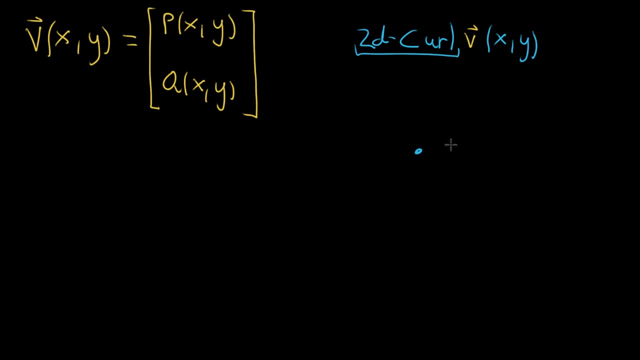 and start to get a feel for it is to imagine the quintessential 2d curl scenario. Well, let's say you have a point- and this here is going to be our point- sitting off somewhere in space, And let's say there's no vector attached to it. 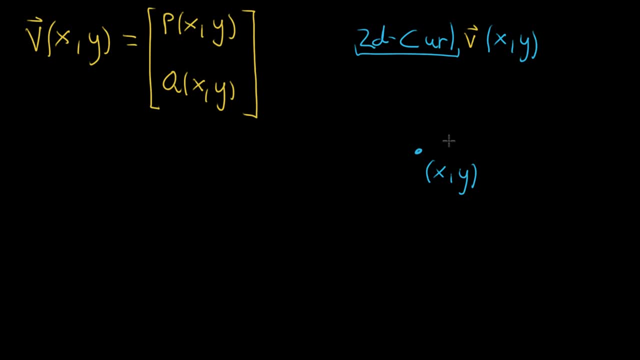 as in the values p and q at x and y are 0. And then let's say that to the right of it you have a vector pointing straight up Above it in the vector field. you have a vector pointing straight to the left. 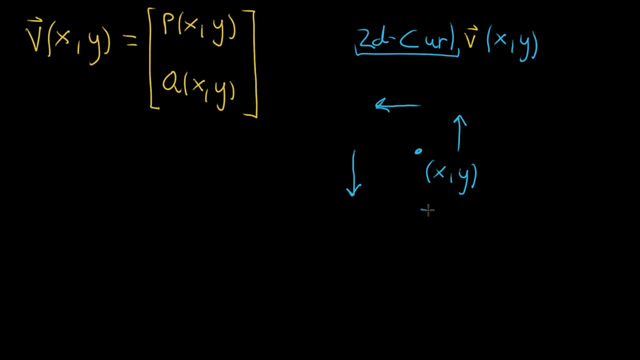 To its left you have one pointing straight down And below it you have one pointing straight to the right. So, in terms of the functions, what that means is this vector to its right, whatever point it's evaluated at, that's going to be q is greater than 0.. 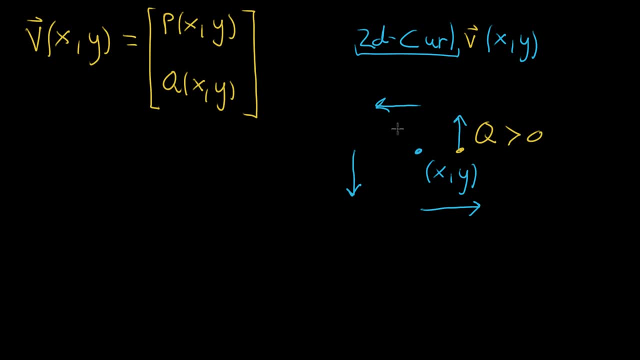 So this function q, that corresponds to the y component, the up and down component of each vector, when you evaluate it at this point, to the right of our xy point, q is going to be greater than 0. Whereas if you evaluate it to the left over here, 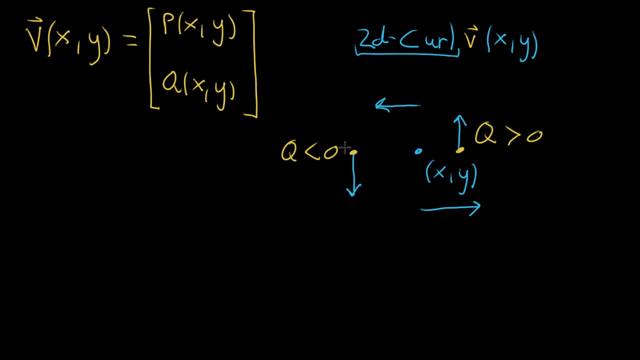 q would be less than 0. Less than 0. In our kind of perfect curl will be positive example. And then these bottom guys. if you start thinking about what this means, for you'd have a rightward vector below and a leftward vector above. 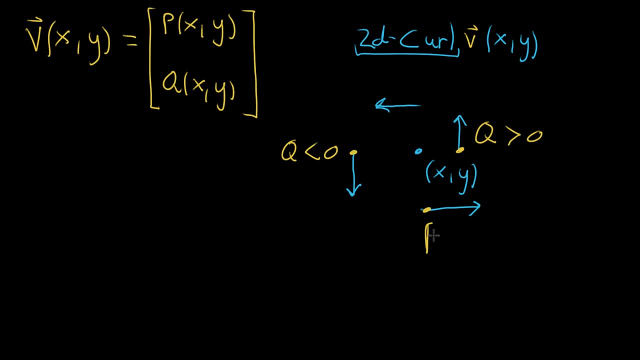 The one below it. whatever point, you're evaluating that at p, which gives us the kind of left-right component of these vectors, since it's the first component of the output, would have to be positive. And then above it, above it here: 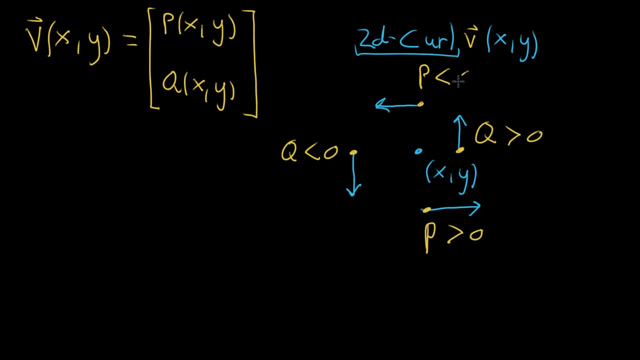 when you evaluate p, at that point it would have to be negative, Whereas p, if you did it on the left and right points, would be equal to 0, because there's kind of no x component, And similarly q if you did it on the top and bottom points. 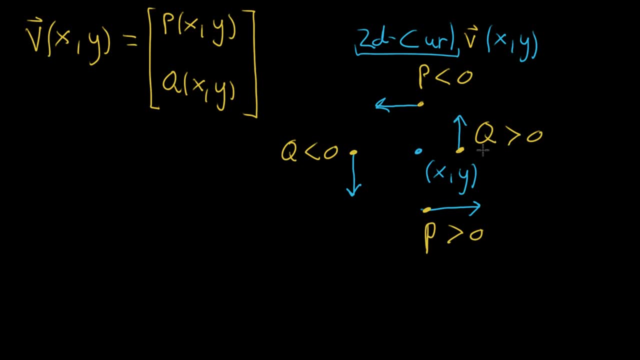 since there's no up and down component of those vectors, would also be 0. So this is just the very specific, almost contrived scenario that I'm looking at And I want to say, hey, if this should have positive curl. 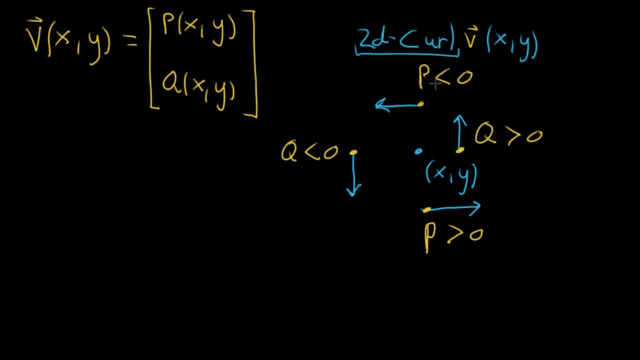 maybe if we look at the information, the partial derivative information, to be specific about p and q in a scenario like this, it'll give us a way to quantify the idea of curl. And first let's look at p. So p starts positive. 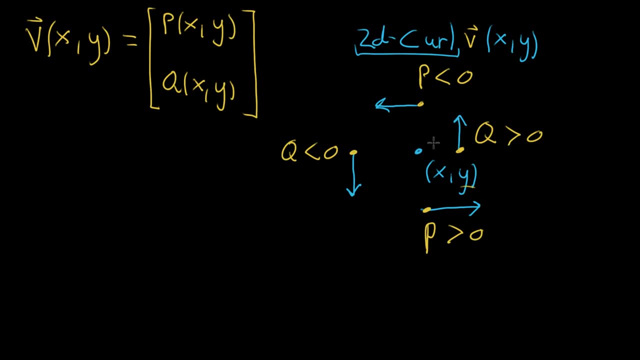 and then as y increases, as the y value of our input increases, it goes from being positive to 0 to negative. So we would expect that the partial derivative of p with respect to y. so as we change that y component, moving up in the plane, 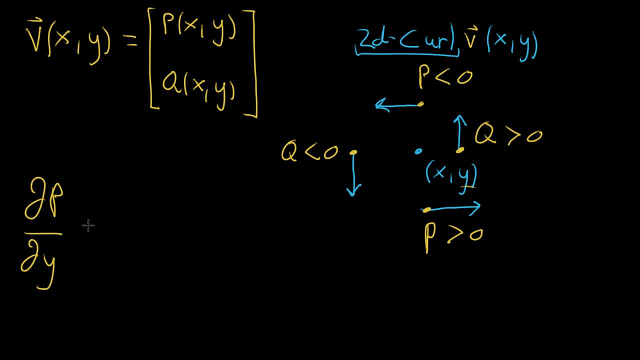 and look at the x component of the vectors. that should be negative. That should be negative in circumstances where we want positive curl. So all of this, we're looking at cases. you know the quintessential case where curl is positive. So evidently this is a fact. 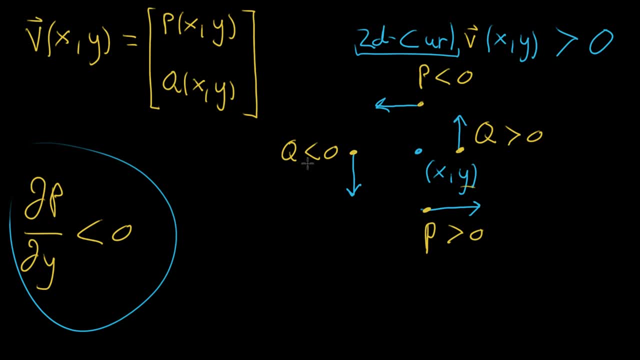 that corresponds to positive curl, Whereas q. let's take a look at q. It starts negative when you're at the left and then becomes 0, then it becomes positive. So here, as x increases, q increases. So we're expecting that a partial derivative of q